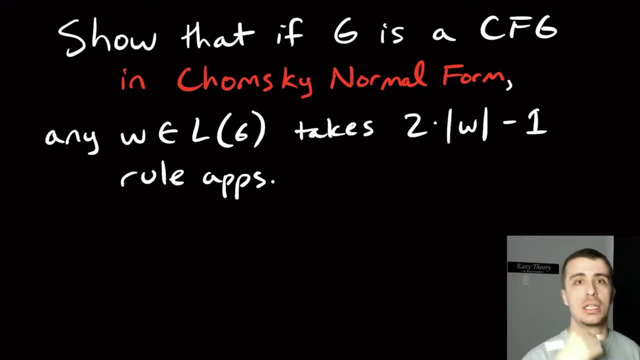 If you don't have a grammar in Chomsky Normal Form, you can't guarantee this. So it's nice that when it's in this form you know exactly how many rules to apply. So this is not actually correct. So this statement right here is true if the string w is not the empty string, But if it is the empty. 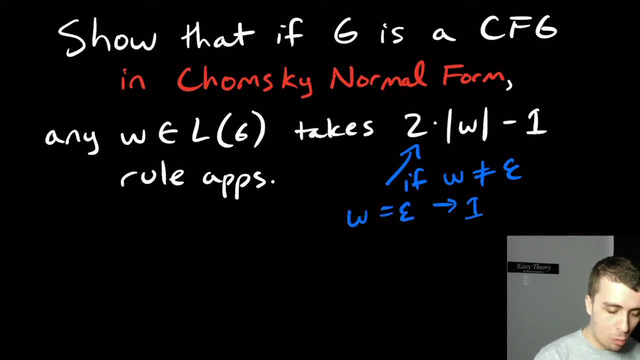 string, then it will take one rule, And so the statement's not true, because two times zero, which is the length of the empty string minus one, is negative one, which makes no sense. So it needs to be at least. But other than this special case, it is two times the length of w minus one. 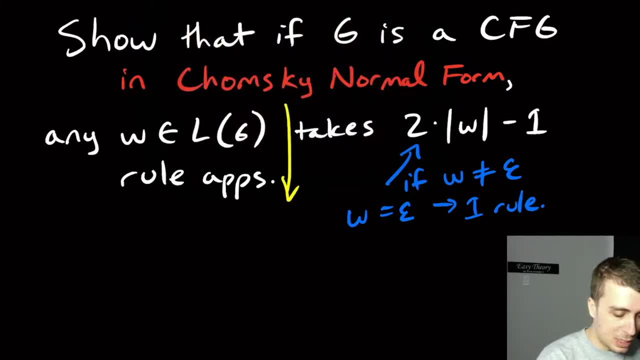 So for those of you who don't know what Chomsky Normal Form is, let's fill us in. So: Chomsky Normal Form. we have three different rule types, So the rules that were allowed are: we can have the start variable, making the empty string and only the start variable. 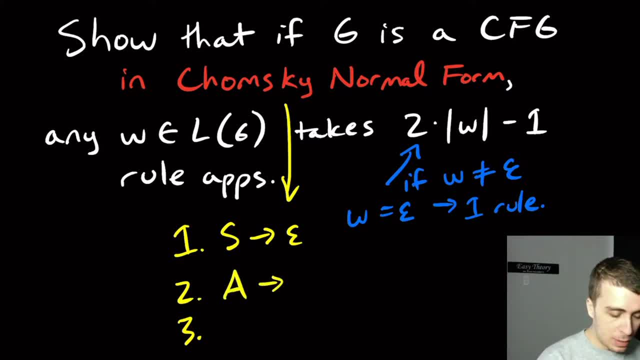 We can have a single variable making a single terminal, or we can have a single variable making two variables, where the two variables on the right side are not the start variable. And on my channel I've done a whole bunch of videos about Chomsky, Normal Conversion and all this stuff. 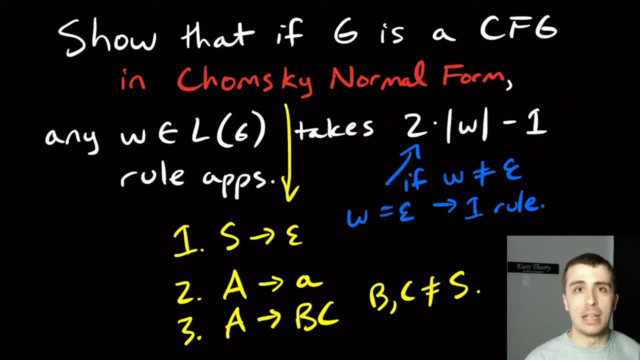 And I've mentioned this fact right here- that we're going to prove here, but I haven't made a specific video on it, so that's why we're here. So I'm not really interested in how to actually get a grammar in C and F. You can always do it. 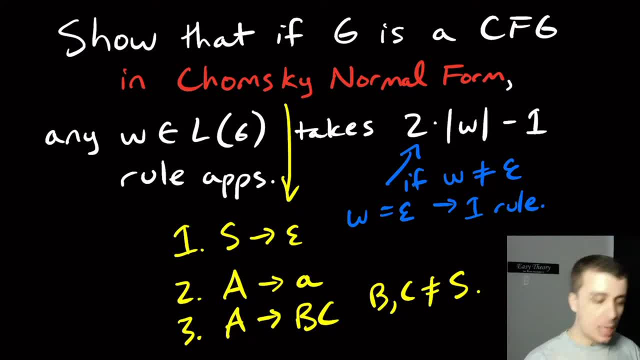 There is a conversion algorithm that always works to do it, But here we're just focused on this question. So here this is saying not that there is a specific way to get to length times the length of w minus one, It's that every way to make any string in the language of the grammar takes exactly that many rule. 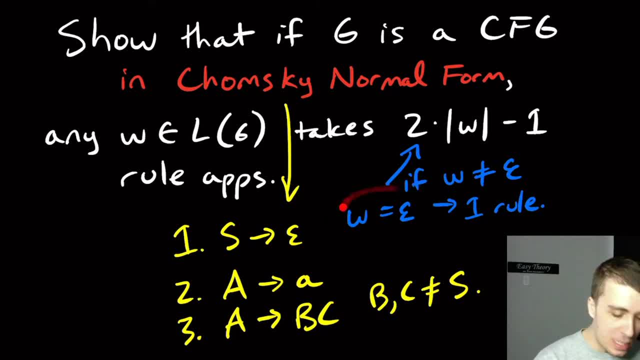 applications other than the empty string. So we can actually prove this exception right here pretty easily, Because if it's in Chomsky Normal Form, the only rule that can exist to generate the empty string is this one, And we can't use any of the other variables down here because they're not the start variable. 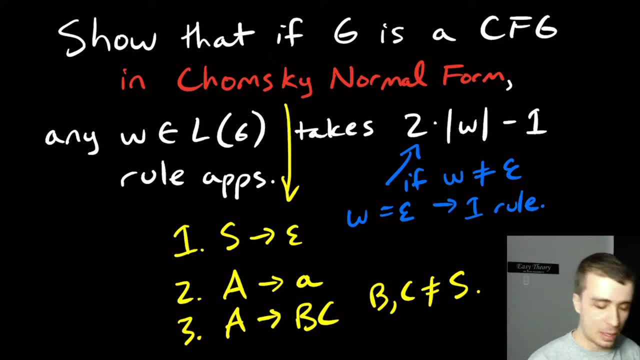 So we can't like come back up here and generate the empty string. So the only way we could ever generate the empty string- if it's in the language of the thing- will take exactly one rule application, starting with the start variable. So this one is a check. 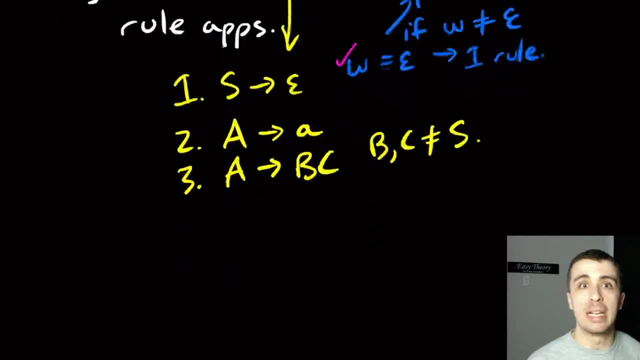 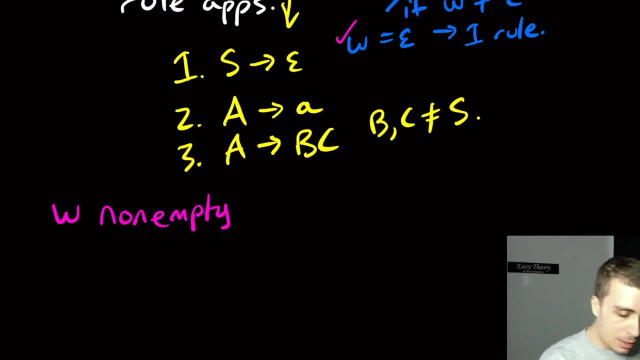 We already know how to do that. So now let's suppose that the string is non-empty. So let's consider when w equals 1.. If w is non-empty, then we have two cases. So what if the length of the string w is exactly 1?? 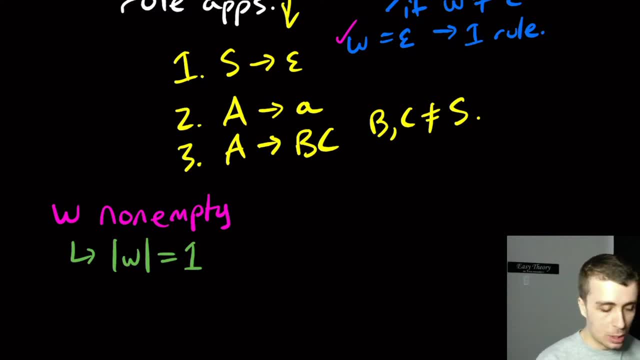 Then if it's exactly one character, then we could only apply this rule right here, Because if we apply this one down here, the two variables on the right side are not the start variable, And so they must generate at least one character each, and so then 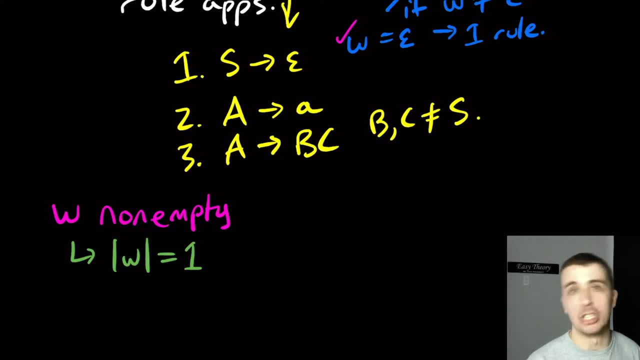 we would be stuck because we would have at least two characters being generated, oops. so we would have to apply a rule of this form, where we have to have the start variable on the left side, but we can have any variable here, but it would in this case have to be the start variable and it makes a single terminal. 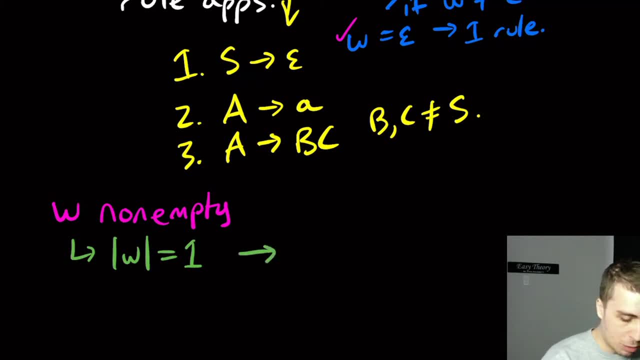 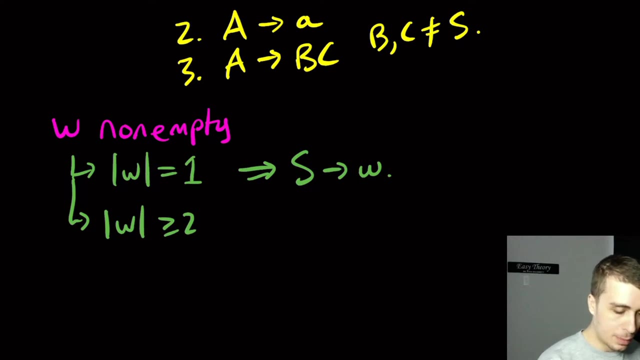 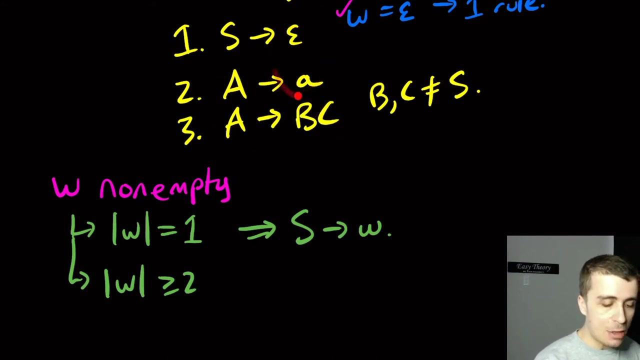 and so that would imply that we get exactly one rule. so we would have S generating W in exactly one rule, and that's one, and that's pretty easy to show. so now let's consider when the length of W is at least two, then we must apply this, this one, right here. first, because we apply either of the other two. 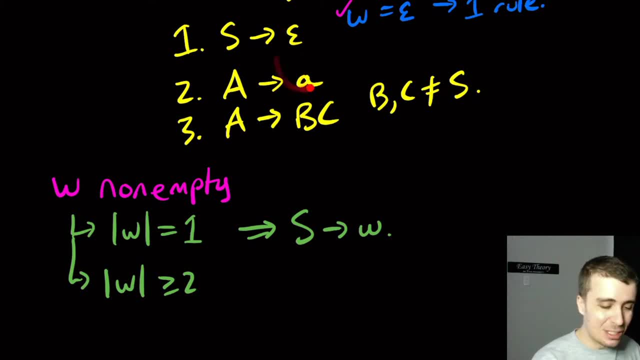 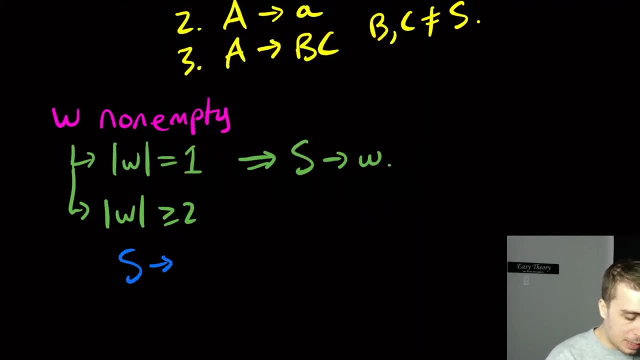 first. then we're stuck because- because there are no other rules to apply once we apply this one. so that means that we started with the start variable and we got BC, and then we replaced B with something, or maybe C with something, it doesn't really matter. and then let's just say: 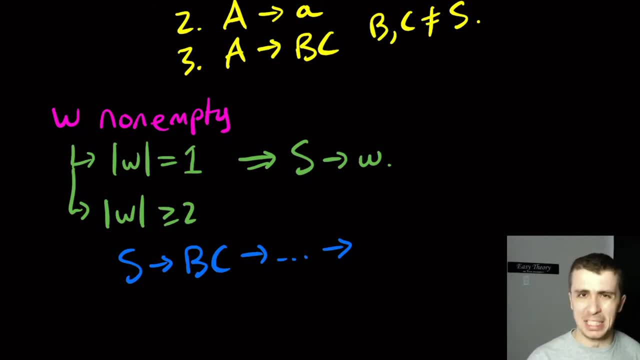 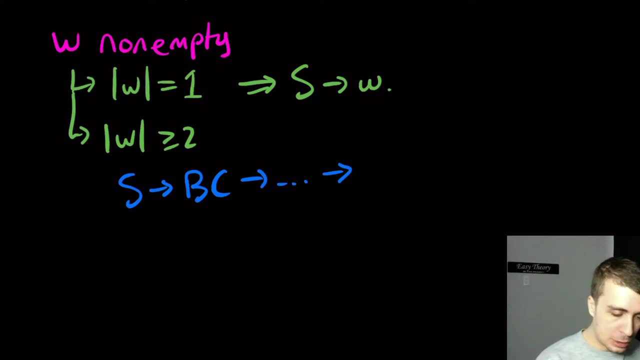 for all intents and purposes, and we'll see why this is sufficient later. look, for all intents and purposes, let's say that we don't generate any terminals right now. so let's say that we have variable X 1, X 2 up to X n, where n is. 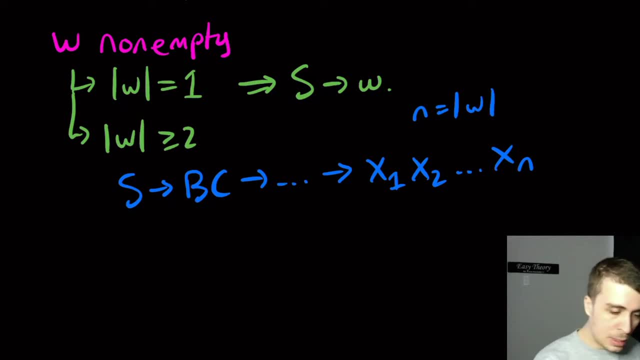 the length of W. so then what we can do is X 1, X 2 up to X n, where n is the length of W. so then what we can do is we can, we can start applying rules of the second type right here, turning each one. 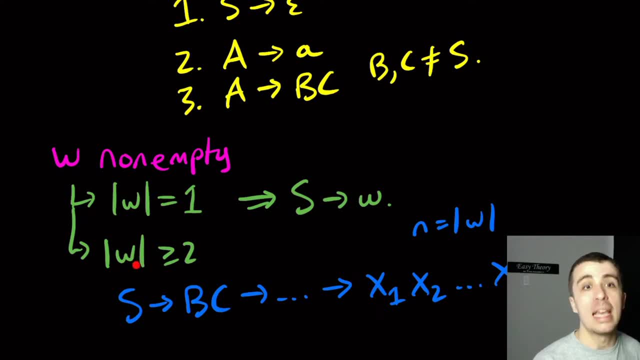 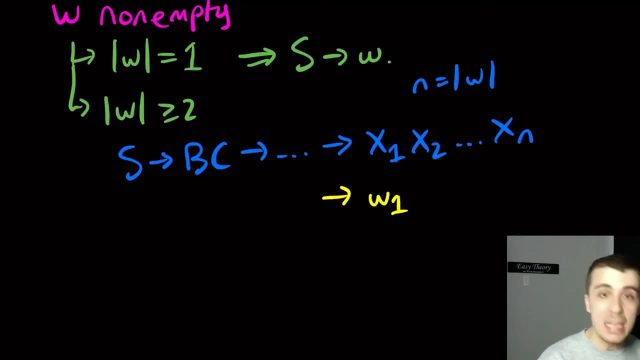 of these variables into the corresponding terminal in the string W that we're after. so I can maybe, for example, convert the first one to be the first character of W and leaving all the others in place, and then we'll convert, let's say, the second one into terminal, and then we just keep going like this. 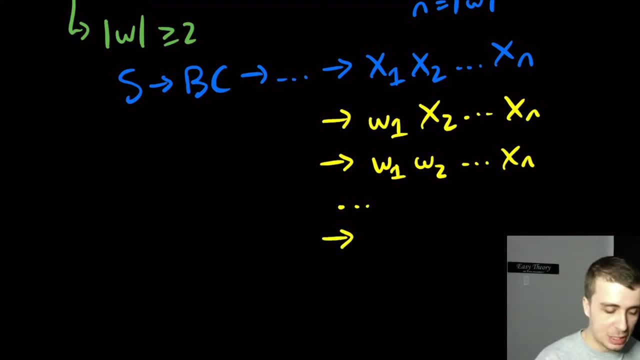 one at a time, because we can only replace one at a time, because it's a context-free grammar, and then eventually we'll get every single terminal like this: we're assuming that the string is in the language of the grammar to start with, so we can actually do this. but so this is certainly one way to do it, but 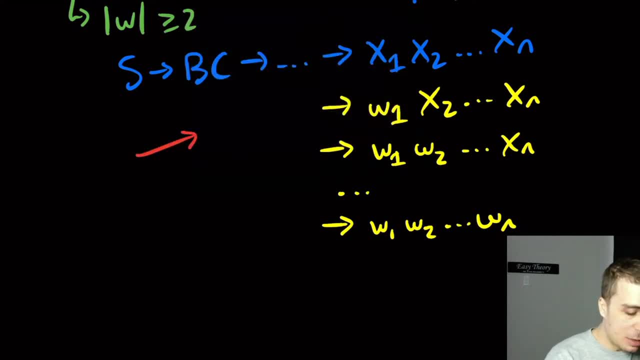 the problem is that this, this derivation, is only one possible derivation, because there are other ones we could choose. for example, if we were to do this with a, for example, we could have replaced the X 2 variable first, or we could have replaced the C instead of the B. over here, there are lots of different. 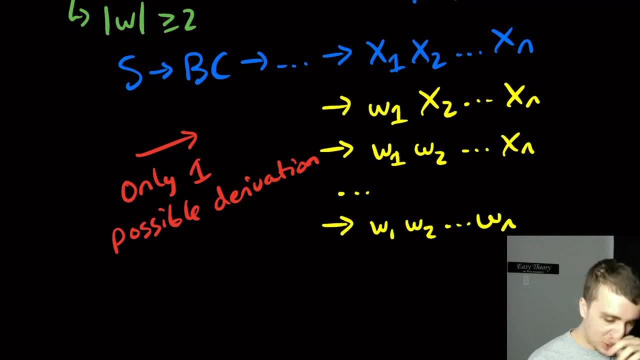 combinations that we could have done. so the question is: this particular derivation you can show takes exactly 2 n minus 1 rule applications, and we will do that in a sec. but we would need to show that this is true for every derivation, not just this one. so let's, it's actually. 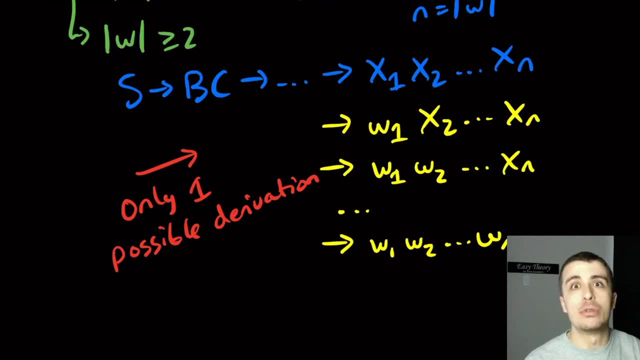 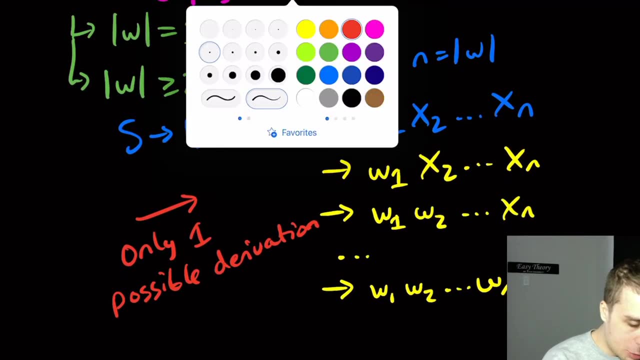 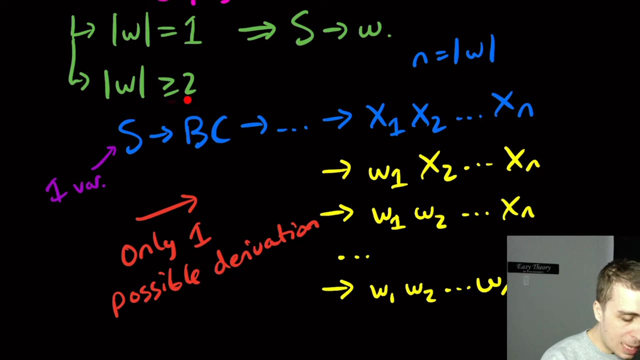 a good idea, though, to make sure that this really is 2 n minus 1, because if it isn't, then then we're screwed. so the way to calculate this is to note that at the beginning, right here, we have exactly one variable and each rule application we. 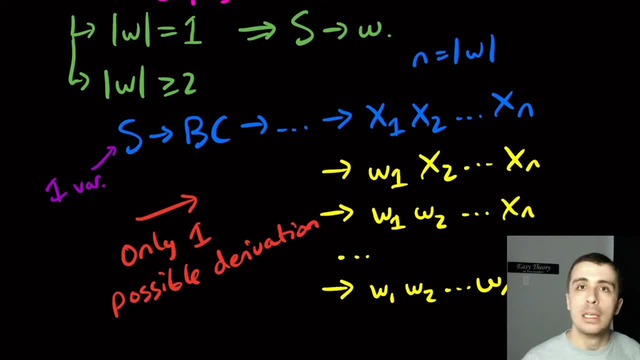 replace this one variable with two. so in each one of these blue rules that we applied up here, we will get an additional variable. so we get plus one, vars plus one, etc. up to we add one more and then we'll eventually get n. so we started with one and then we added one over and over and over and 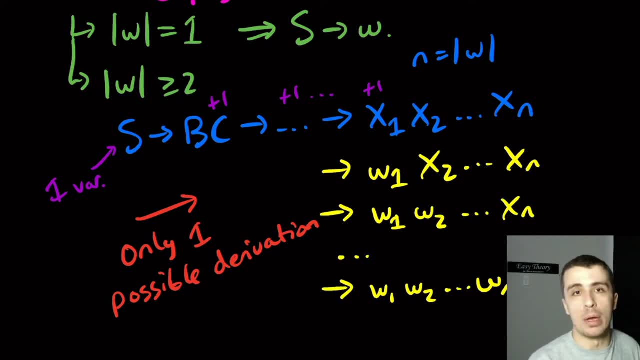 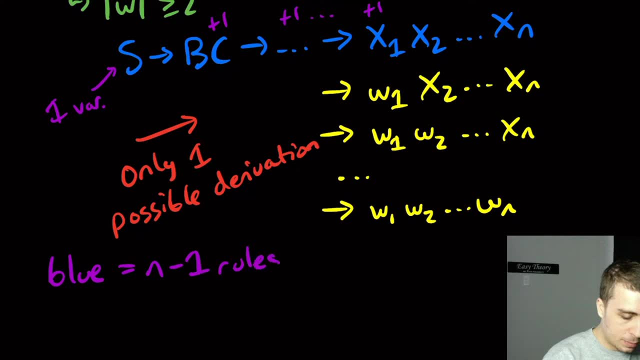 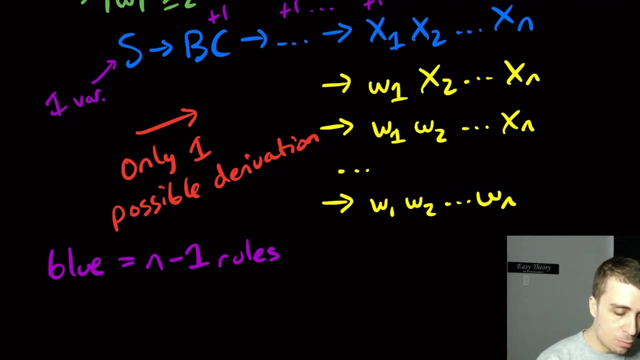 over until we got n, and that takes n minus one rule applications. so the blue rules are gonna be n minus one rules to get there, and then the yellow ones down here. what happens here? well, we can only replace one of the variables with the terminal at a time, and because there are n of them, it would take at least n rules. 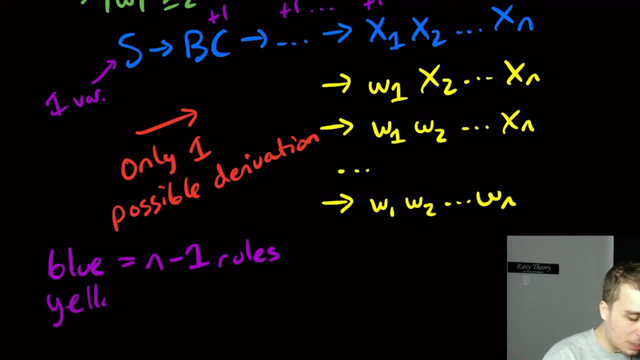 to do that and in fact exactly n rules. so the yellow ones down here are gonna be exactly n rules, and so obviously the total is 2 n minus 1, so that's not hard to see. so why is this true in general, then, not just this derivation? so here's. 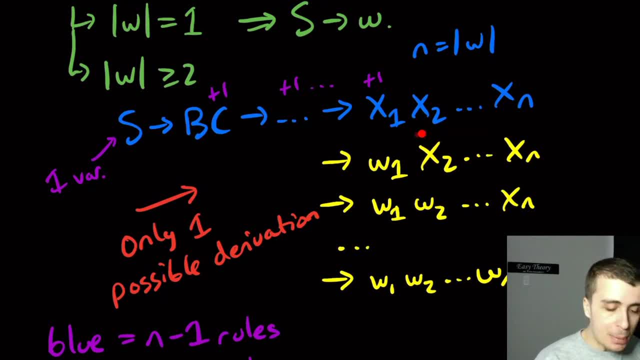 the reasoning. so you have to know that there are n rules and there are rules in the derivative. so you have to be able to generate these n variables at some point of throughout the derivation. it's maybe we do them at the beginning, like we do here, or later, but at some point we must have all n variables generated in some. 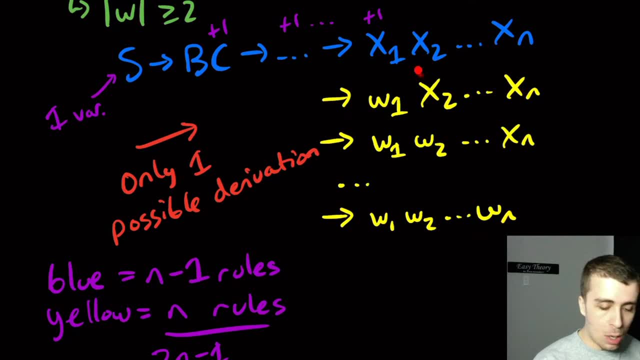 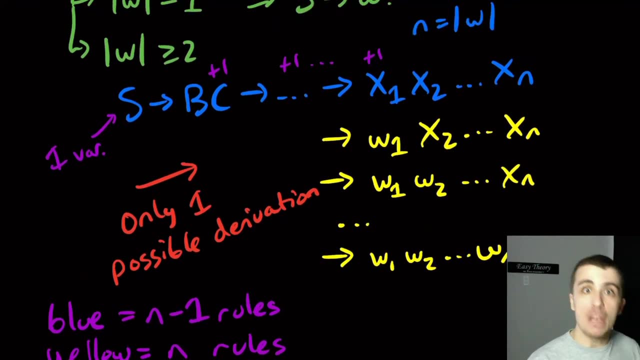 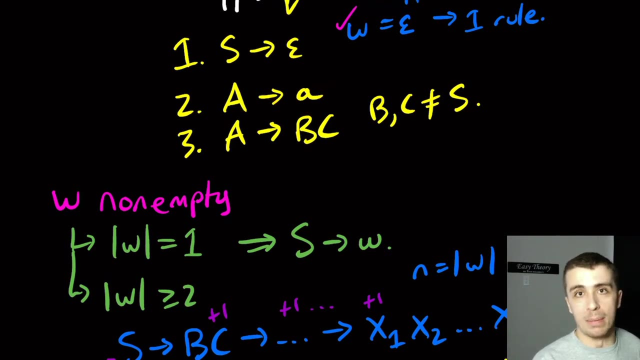 way, and we must have all of those n variables turned into terminals. why must we have all n variables? because if we have fewer of them, then that means that if we have fewer we can only make one terminal out of each one of them, and so we can't make. 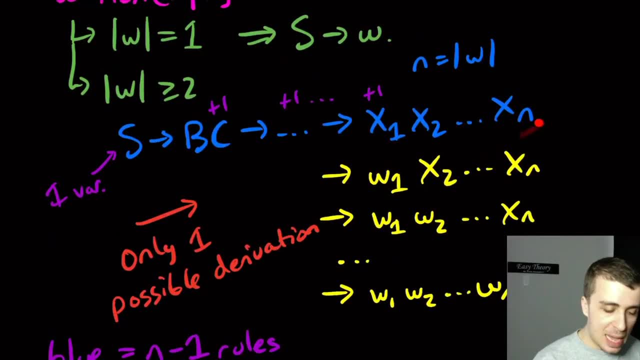 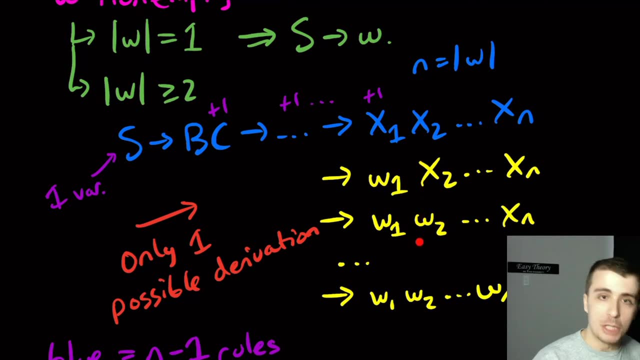 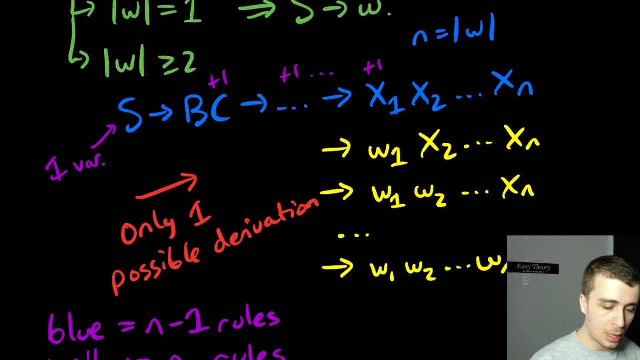 the string itself. so we must have n variables. maybe some of them are the same, but we have n occurrences of variables and each one of them must be converted into a terminal at some point, maybe now, maybe later, but at some point they must all be converted. so that means that we've got to get from one variable to n. 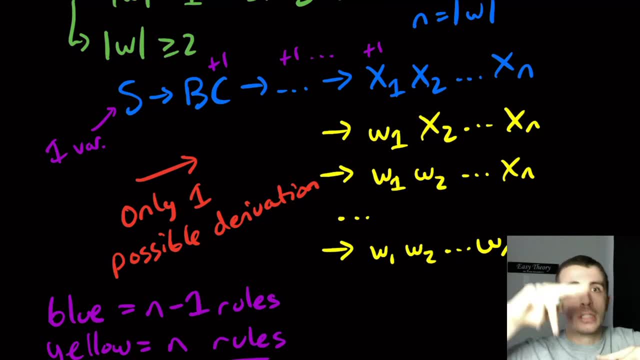 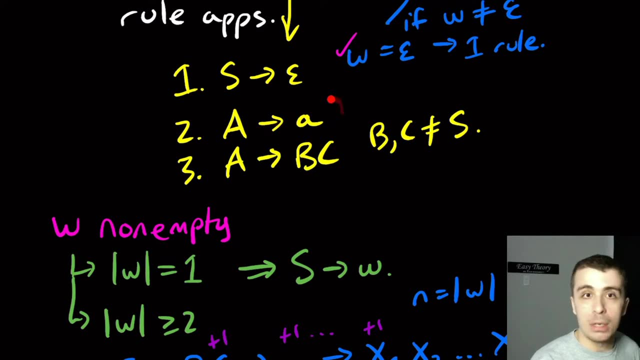 at some point, and we can't mix and match the two types of rules because they're fundamentally incompatible with each other. this one converts a variable to a terminal and doesn't make any variables. this one, uh, adds one variable, but it doesn't make any terminals, so there's no way that we can mix and match them here. 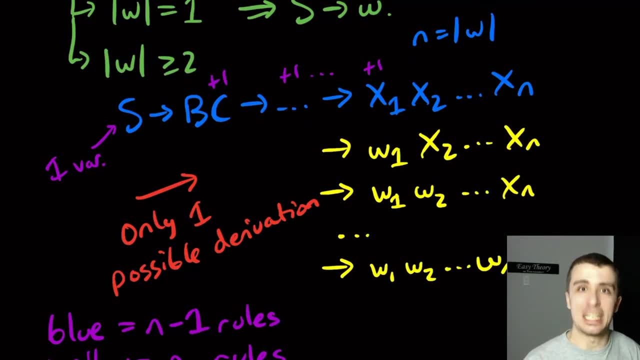 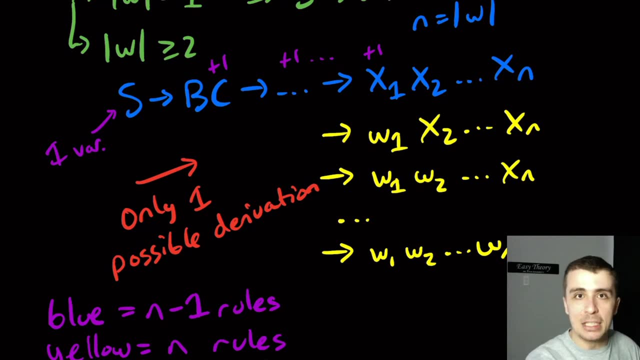 so these two types of rules are entirely distinct from each other. so therefore, we know, now know, that we must have at least n minus one rules, and in fact exactly n minus one rules to make all the variables needed and n more to convert all of those variables into the corresponding terminals.